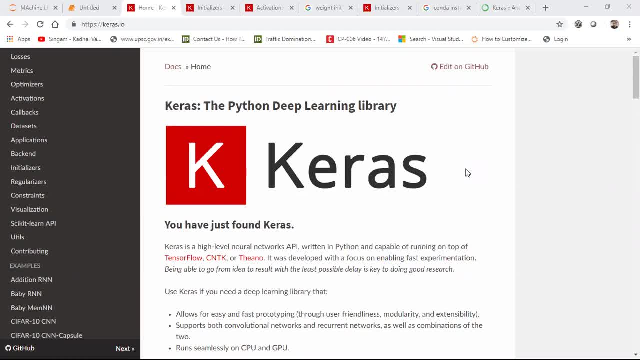 gets updated. what is the initialization techniques of the weights? Now, many people were asking when we will be starting the practical application. Today is the class we are going to start and we will be focusing on implementing everything from scratch in a wonderful way. Unless and until you have understood the theoretical concepts, it will be very, very easy. 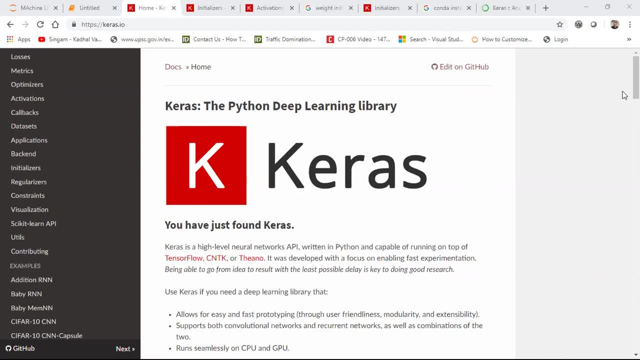 for you to understand everything. So, to begin with, first of all, I need to introduce you to Geras library documentation Everything. it's just like an OSFET database. It's just like an OSFET database. It's just like an OSFET database. It's just like an. 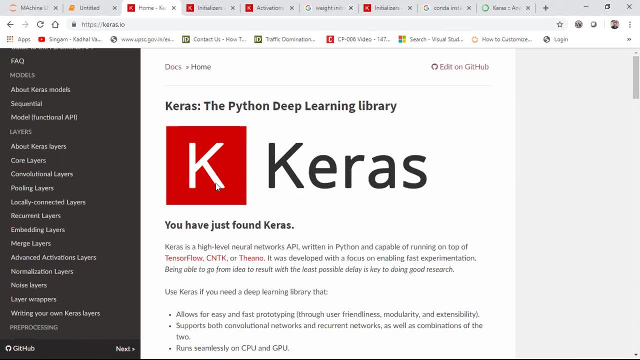 OSFET dictionary. You know OSFET dictionary for implementing your deep learning models And any queries that you basically have. you should come over here, You should try to see over here, because every information is given in this particular documentation itself And, as I go along with the videos, I'll be showing you how you can find out simple details whenever. 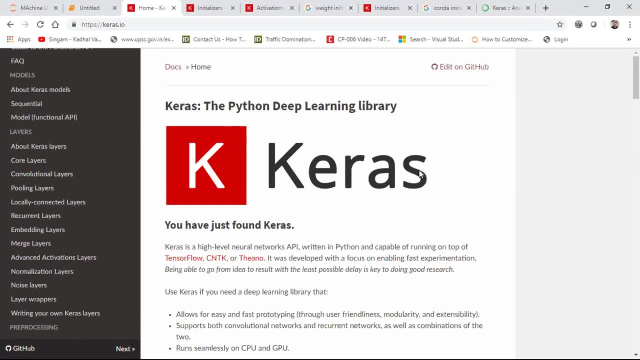 you're using any inbuilt functions. This Geras library is basically a wrapper on the top of TensorFlow or Theano. You can basically use a Theano C and D. These all are open source libraries. It's very, very good for creating your neural networks. 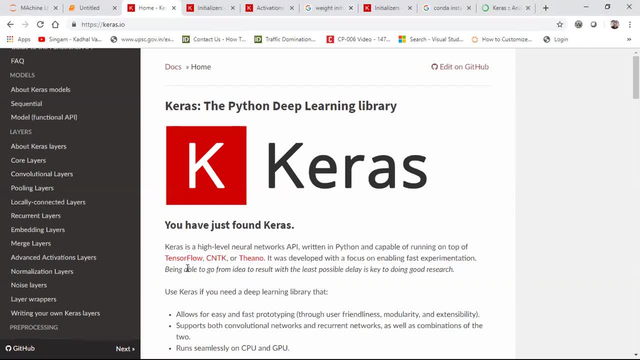 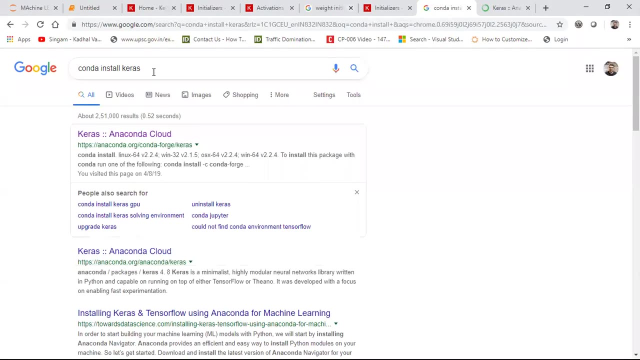 You know, TensorFlow is basically, you know, open. Basically, it is a library that is provided by Google. So let us go ahead and, first of all, try to understand how to install Geras. So, in order to install Geras, all you have to do is that go into Google and write. 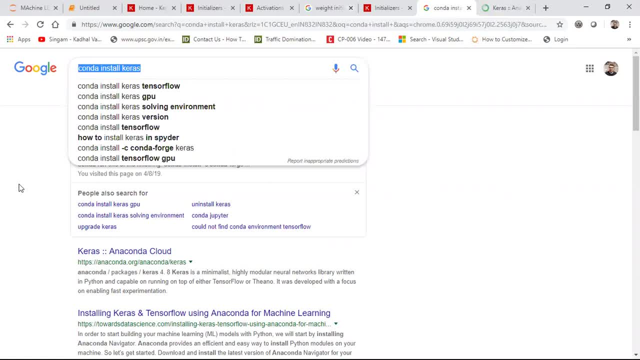 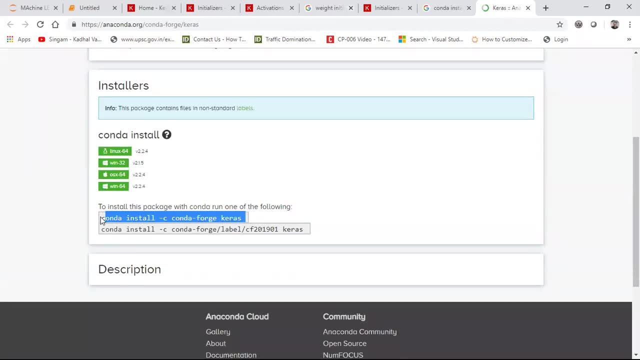 conda: install Geras. As soon as you write the first link that you will be getting over here, just click this. just go over here below, just copy this whole command and just go to your anaconda prompt and paste it over there right. Go to your anaconda prompt and paste it over there. 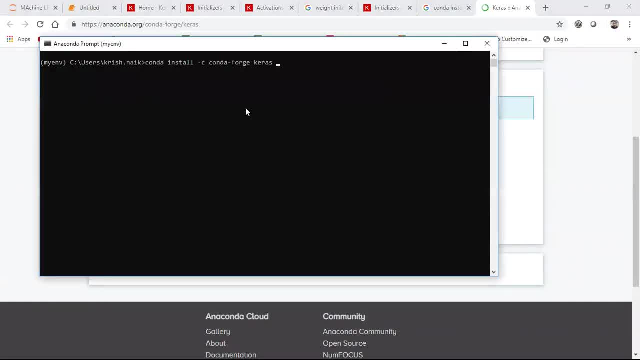 So I'll just go over here and paste it over there. okay, There it is, I'm going to paste it. It will take some time to install this forge. what it makes is that it all the all the other libraries that are dependent on Geras will automatically get downloaded. So after the downloading is completed. 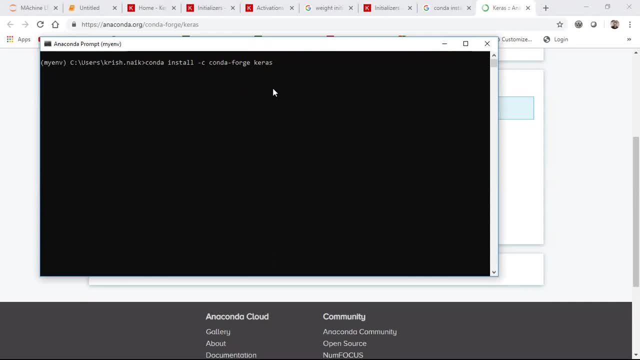 you have to wait. it will take around 10 to 15 minutes for the downloading to happen. Once it is done. now we'll focus on creating a wonderful application which is like a churn modeling data set for a bank customer. We'll try to create a model with respect to that. 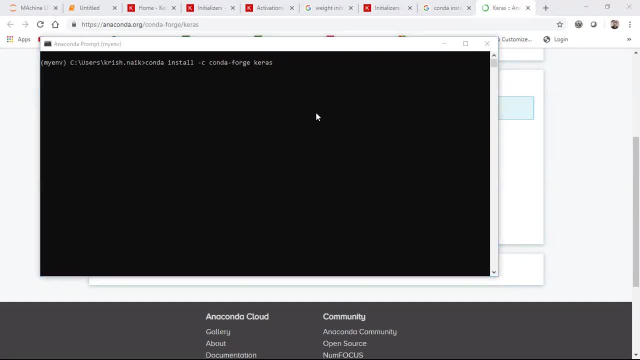 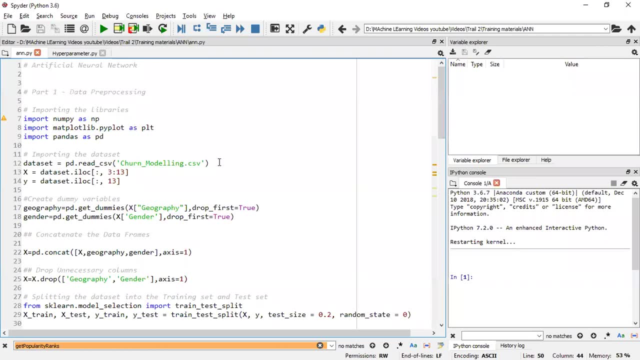 particular data set by using artificial neural network. Let us go back and let me show you the data set how it looks like. So this is my code. First of all, my data set name is churn underscore modeling dot csv. Uh, this particular data set. you can download it from Kaggle Apart. 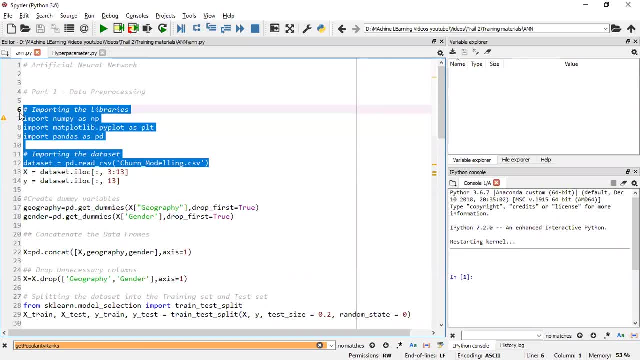 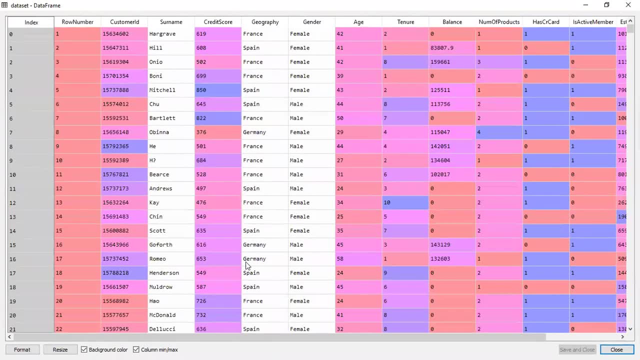 from that, I'll also give you this particular data set in my github link, So let me just read this. I hope everybody's familiar with how to read it. So this is my data set. I'm just going to show it to you. My data set basically has 13 features. Okay, my dependent feature is the. 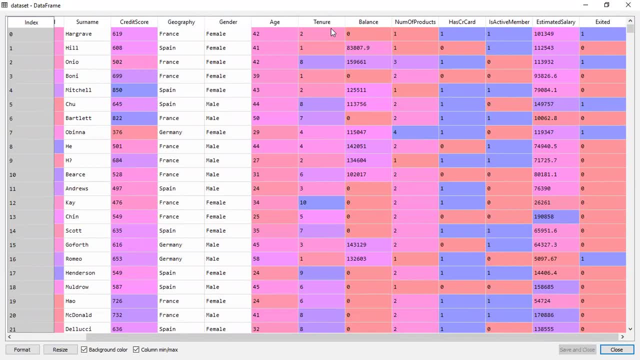 executed column and you have all the other features like geography, gender, age, tenure, balance, number of product as credit card. In this, the dependent feature is your exited it. so the main thing about this particular data set: we need to predict customers in the bank who will be exiting in the future or not. whether they will exit the bank in the future or not, because 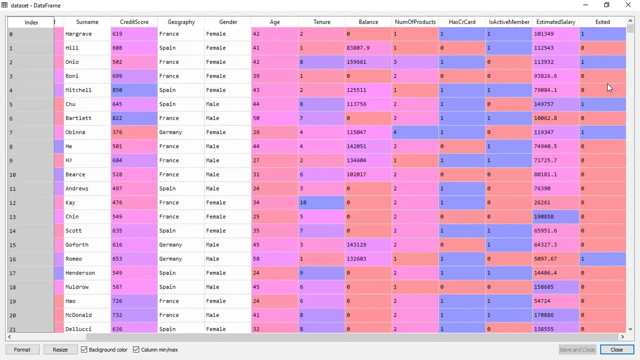 now this churn modeling can play an important role for the bank people, right, because bank wants to, do not want to leave his customer like that, right. and if it is able to predict whether the customer will be leaving the bank in the future, it can provide some better product so that the customer 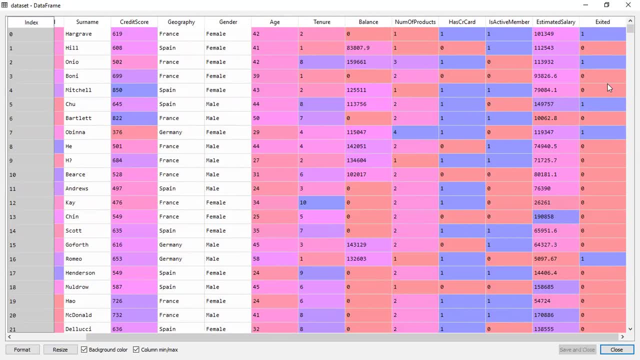 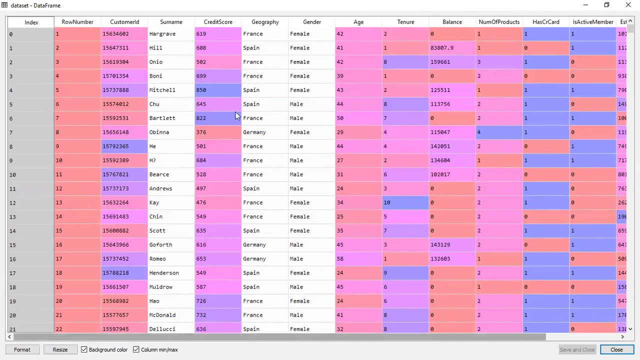 stays in the bank itself, right, so just to bring some loyalty factor. so in this particular data set you will be seeing that first of all we'll see what are my dependent independent features. so i'll be considering all the features from credit score till the estimated salary as my 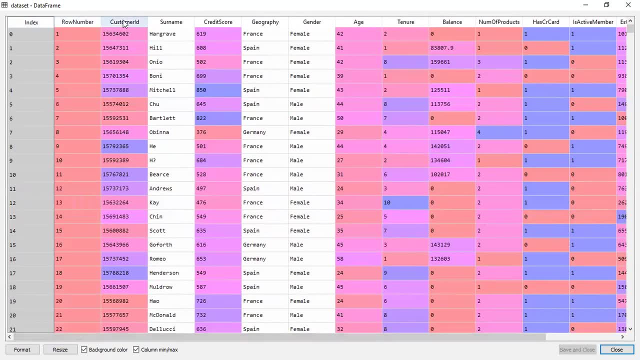 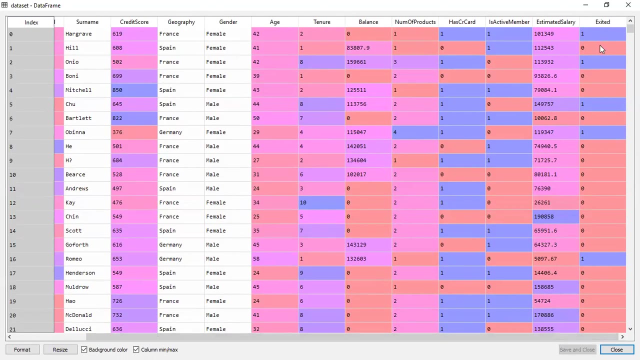 independent features. i will not be requiring features like a row number, customer id and surname, because these are just unique numbers and surname. it is not related to surname, so this one play a very big factor. okay then, my dependent feature is basically my exited column. in this particular exited column, i'll be 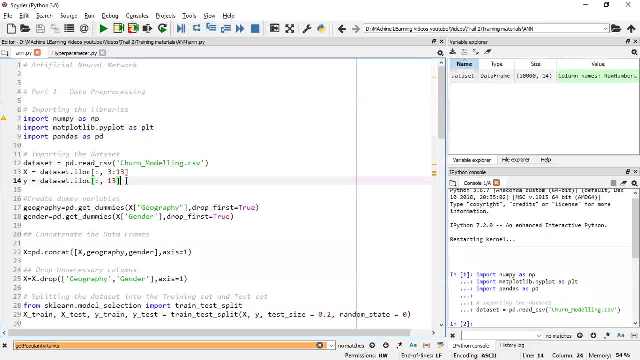 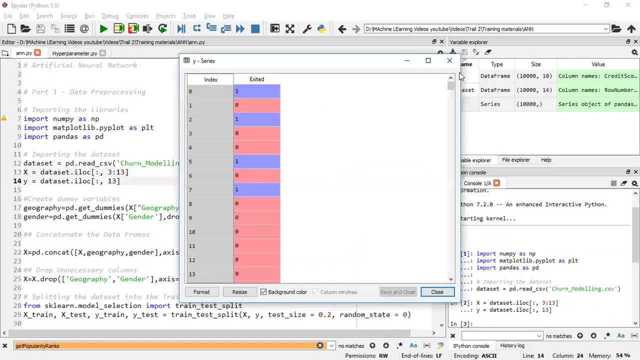 taking my dependent feature. so i'll be using iloc and i'll be creating my independent and dependent features. let me just execute it. it has been created. here is my x data set and here is my y data set. now, remember, guys, in my data set you have seen features like geography and gender. 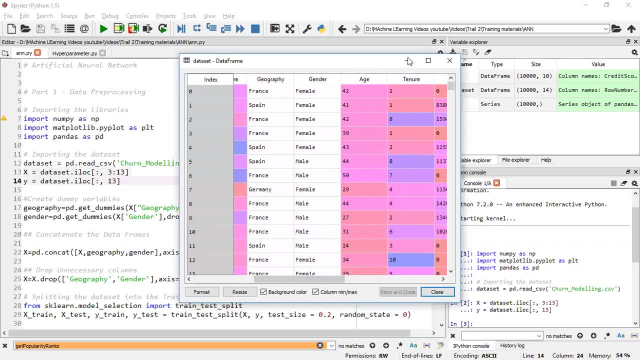 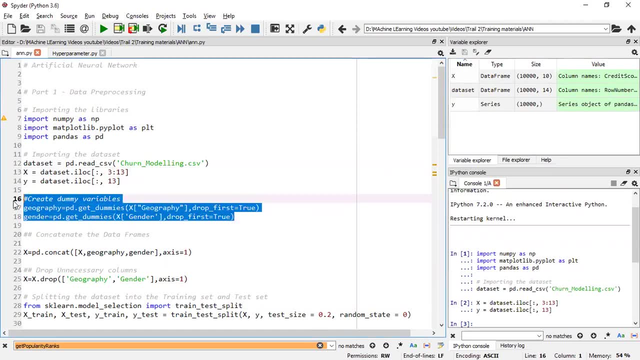 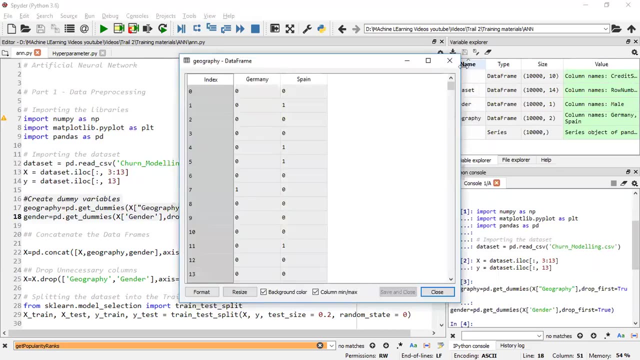 these features are basically category features. right, we need to convert this into dummy features and for my previous videos also, i'll be using get underscore dummies to create the dummy variables. so i'll execute it. all my dummy variables gets created. it's stored in this particular gender and geography data frame. okay, now what i'm going to do? i'm going to concatenate. 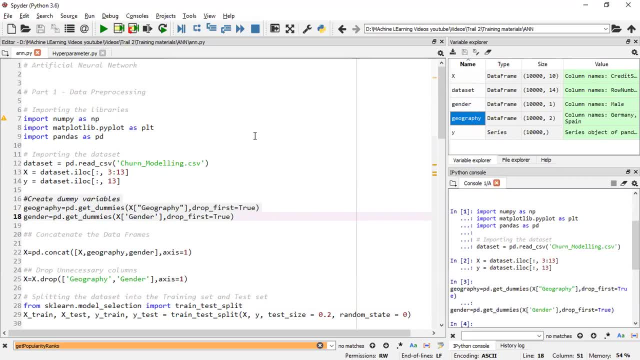 this with my x data set. okay, because x is all my independent features and for concatenating, i'll be using pd, dot, concat and x, geography and gender. x is equal to 1. so i'll just execute it. so x- all everything- is getting concatenated. you can go at the end and you can see that three features. 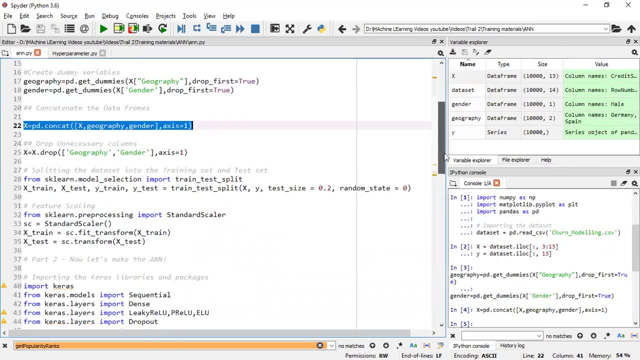 has been concatenated that in it- that what we are going to do is that we are going to drop the geography and gender column, which was my original category of columns, because I have converted that into dummy variables, right, so I'm going to drop it. for dropping it, I'll basically use X dot drop my column. name is geography and 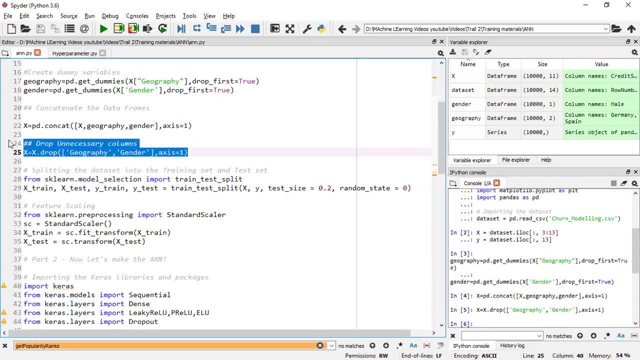 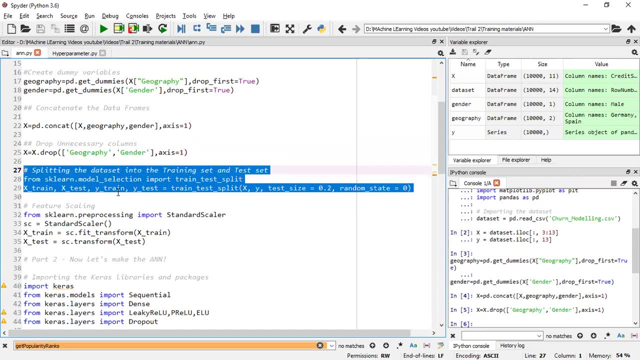 gender. so let me just drop this. are dropping unnecessary columns. and then, finally, I'm doing a train test plate. I hope everybody is familiar how to do a train test plate. by using a scale on our model selection, you're using the library called a strain test plate. once you apply this, you'll be able to do the 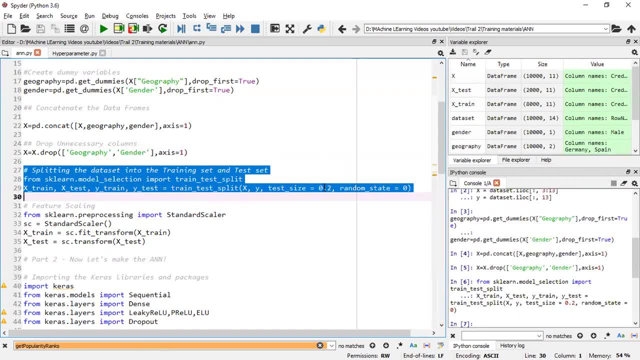 train test plan, and here I'm basically giving the test sizes: 20%. okay, so this is. your extreme is basically having 8,000 records. the total number of records are 10,000 days, so you'll be able to implement it very nicely, oh the. 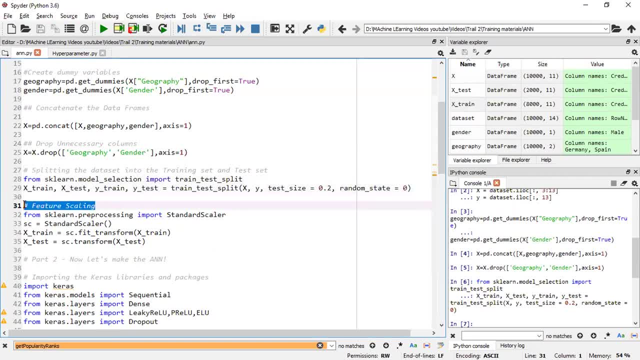 next thing is that: whether do we require feature scaling? I also also ask this question in at one of my previous video, where I think just randomly put some deep learning videos right. that time I had asked whether you require feature scaling in standard scale or feature scaling in. 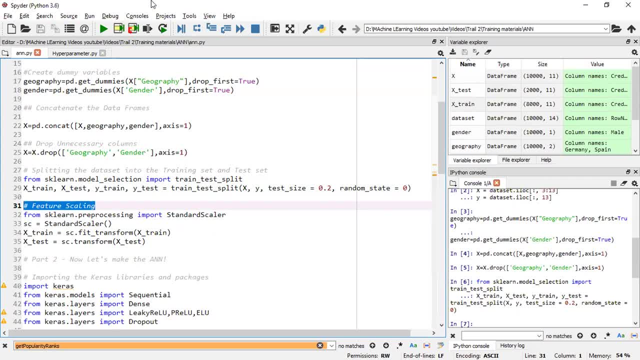 deep learning or not? so the question, so the answer is obviously will require feature scaling, why. I'll tell you, as you know, if I create a deep neural network from my theoretical classes. right, suppose, this is my input layer, this is my hidden layer, and finally I have my output. remember, this is my feature X 1. 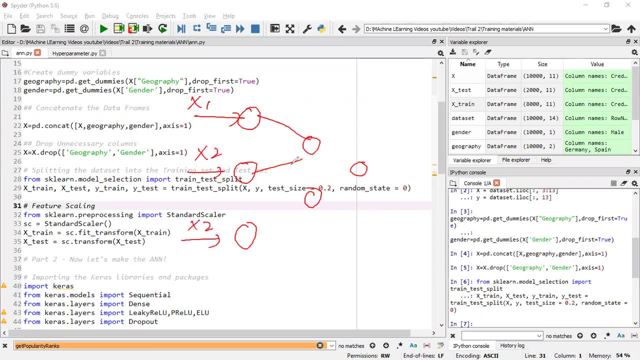 X 2 and X 3 right and, as we know that it is connected to all the hidden neurons right, disconnected to all the neurons. and here you initialize weights. now, always remember the first step is that this inputs gets multiplied with the weights right. so I can write it as summation of: i is equal to 1 to n w of. 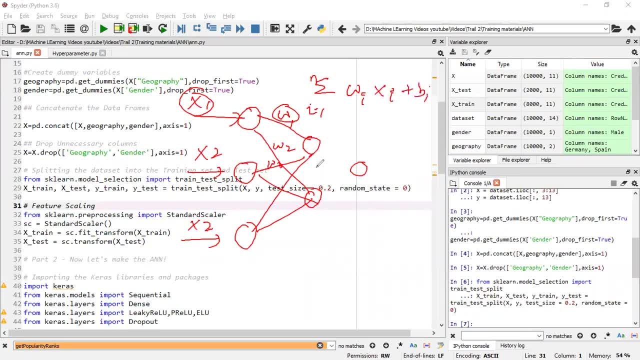 i, X of I right plus the bias right bias will be added over here: b1 and b2. now remember this particular step is also very important. how much time it is taking. now suppose if my magnitude of X, 1, X, 2, X, 3 is completely. 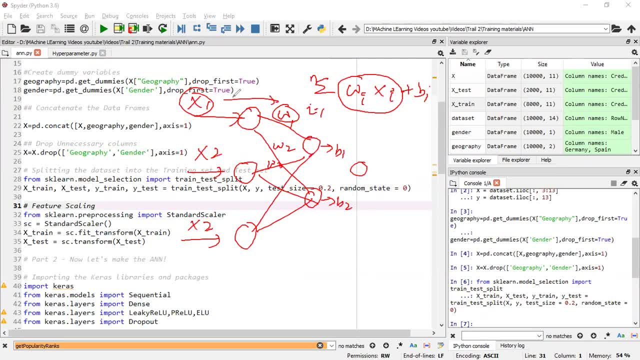 different. you know, it is a very high number, so this multiplication usually takes time. so what we should do is that we should try to scale down all these features in the same scale range in the same scale range. once we do this, what will happen is that the multiplication will happen quickly and when the back 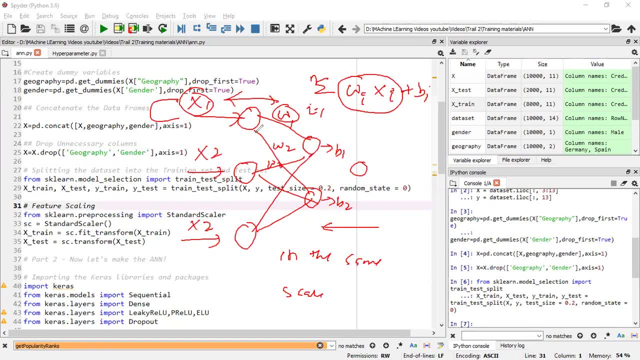 propagation is also done. the derivative of the weights can be easily found out for a smaller numbers. so, because of this, what will happen? the gradient descent curve right, the convergence will happen quickly, the global minima point will. we will be able to find out very quickly. so let us just go and you know. and 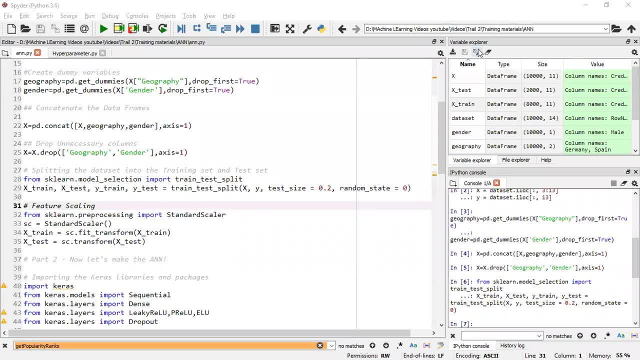 dissolve things we have basically discussed in the deep deep learning playlist, theoretical class also, and in my previous videos also. so what I'm doing is that I'll basically use feature scaling for that. I'm going to import a library called a standard scalar and then I'm doing fit, transform my train. 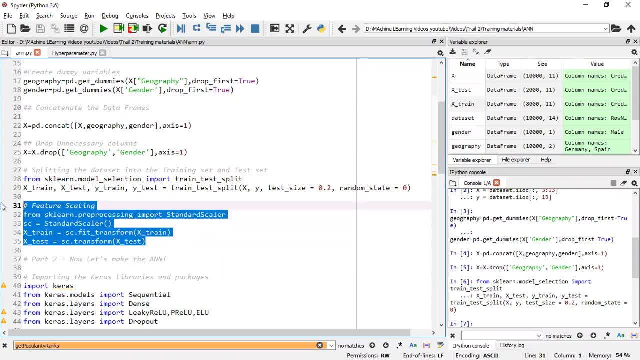 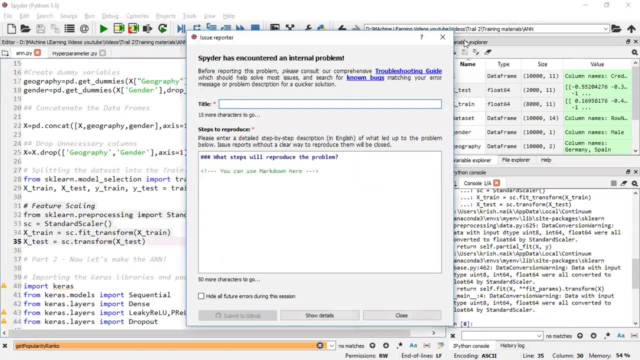 and transform on my test. I'll just execute this. as soon as I execute this, you can see my X test and X train has become floating data and all will be in the same scale. if I just go and execute my X train, you can see that it. 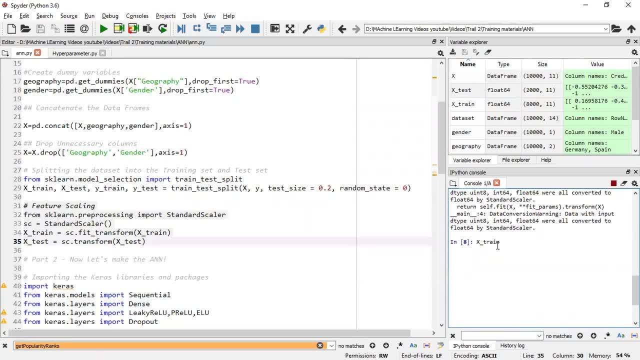 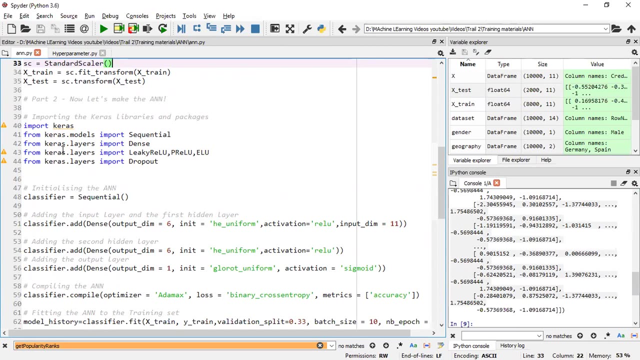 will be in the same score train here. these are just areas of numbers and it will be basically be in the same scale. now the main thing is that let's start making the ANN. so for creating the artificial neural network guys, there are some very good libraries required. of the library that I've had I'm basically using 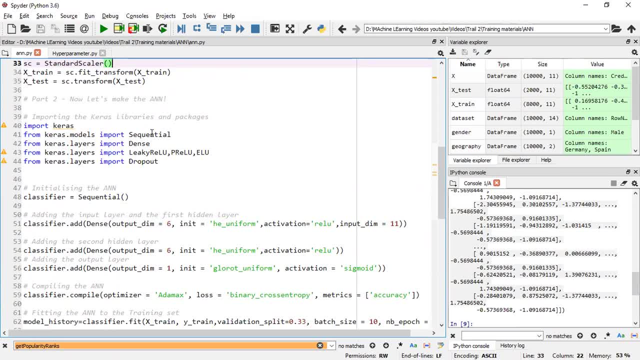 is carers in carers. first of all, you need to import the models. so every model, every neural network that you create, whether it is an ANN, whether it is information in the network, whether it is in record, a neural network- you have to basically import the sequential library. sequential library is: 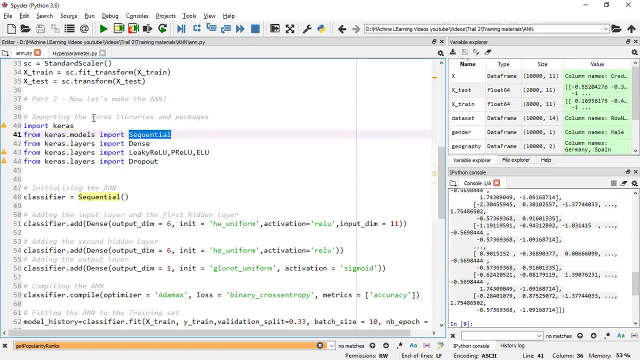 responsible in creating this kind of neural networks right then. after that, any hidden layers that you need to create at that time, you will basically be using this dense library and for that you'll be importing from Keraslayers and then you can also import different kind of. 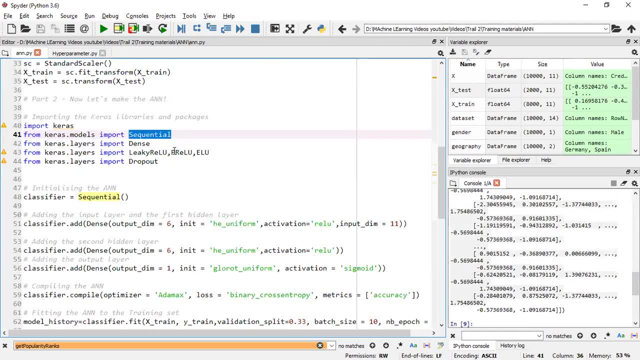 layers like, which is basically an activation function, and other type of value functions- Not important this particular statement right now, but later in the upcoming sessions I'll be discussing about them more. And if you want to also import a dropout layer, you can do that. 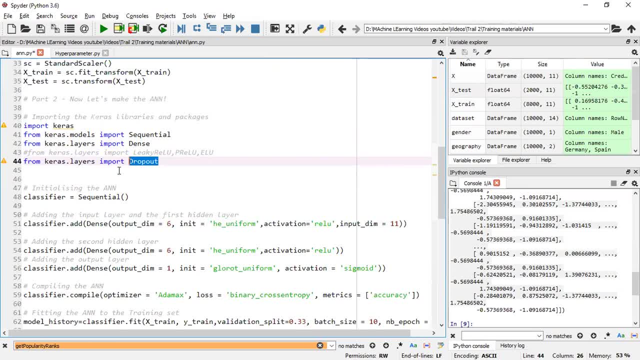 You know that what is dropout used for? You know dropout is basically your regularization parameter and you'll be using them more frequently whenever your neural networks are quite deep. But first, to begin with, what I'm going to do is that I'm going to import all these particular libraries. 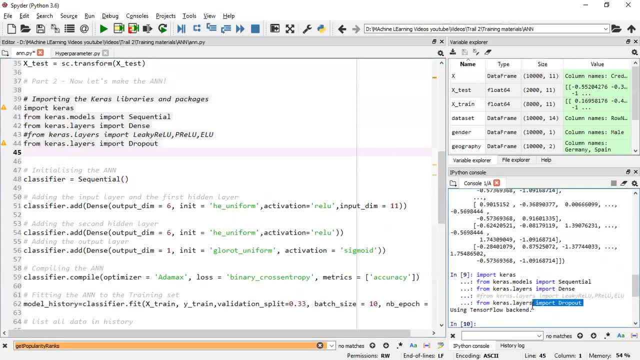 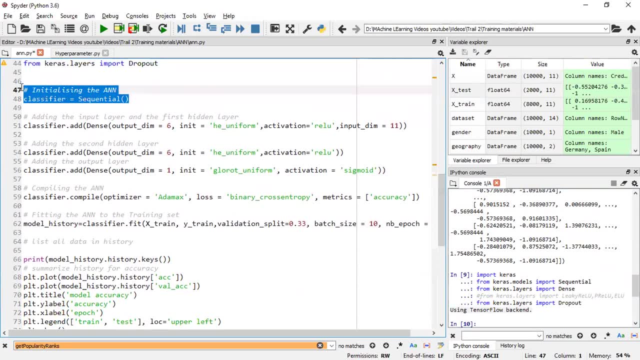 After my import takes place, you can see the message saying that using TensorFlow as the backend, because that is how my libraries got installed, And then first I'll initialize my sequential library. So here it is. This will be an empty- you know empty- neural network. 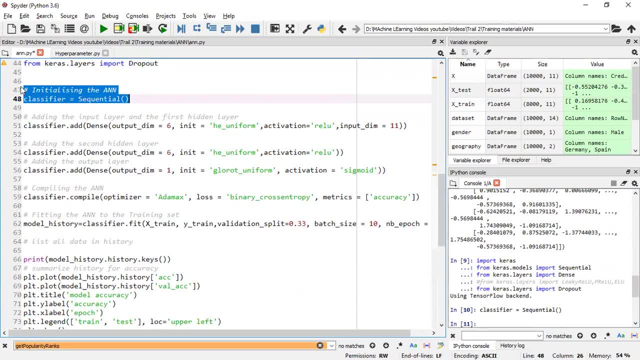 currently, You know that, how many hidden layers will be present and how many neurons are present over there, And then I write classifieradd, and now I'll be using the dense layer to create my first hidden layer. In this, my first parameter will be my. 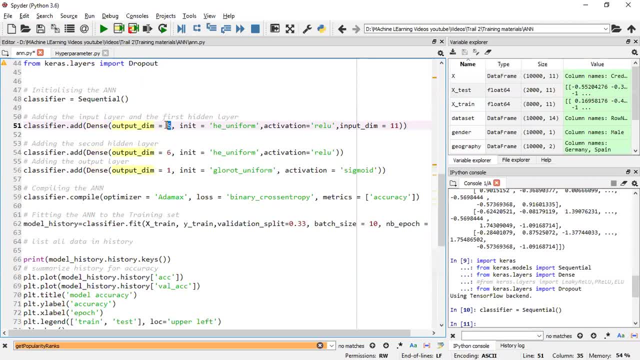 output dimension. The output dimension is basically, I'm saying that in my first hidden layer I'm going to consider six hidden neurons And this is basically initialization parameter. This basically indicates that how your weights needs to be initialized. So here, always remember guys, ReLU activation whenever you're using. 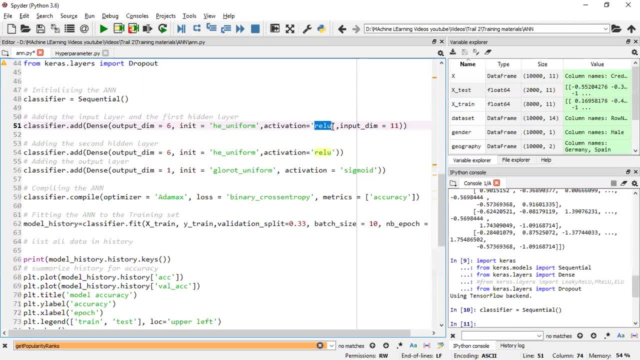 a ReLU activation function. In my theoretical classes in deep learning, I told you that whenever we are using ReLU activation function, the initialization weight initialization, called as heUniform and heNormal- works well. So in this case I'm basically taking heUniform and the last parameter that I'm providing. 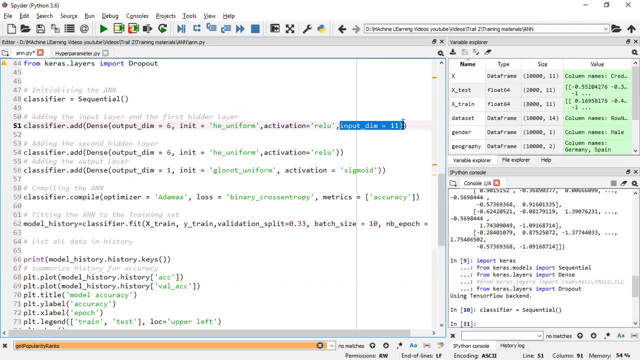 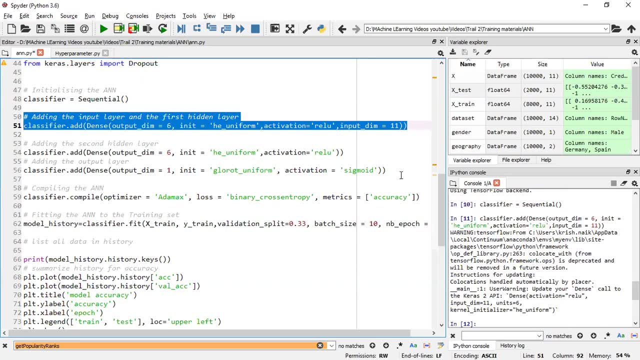 is the input dimension. But remember, guys, this is with respect to Keras 1.0.. Now Keras API has also got updated. Let me just execute this. You can see, as soon as I executed this, I got some warnings right. warning basically says: 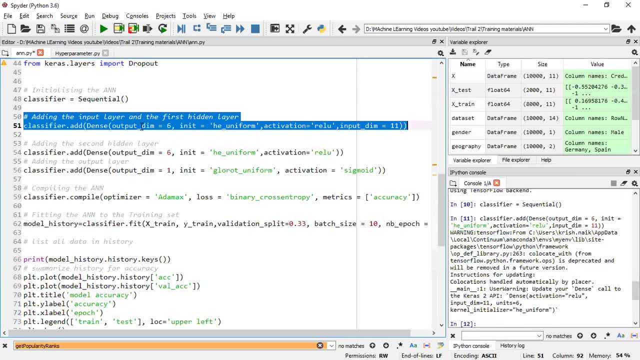 that now your output dimensions- right, output dimensions- has been converted into something called as units. I'm going to put units over here, right? Similarly, my initializes initializer is basically converted. the keyword is basically converted into kernel initializer. I'm going to replace that So you can see over here. right now I have. 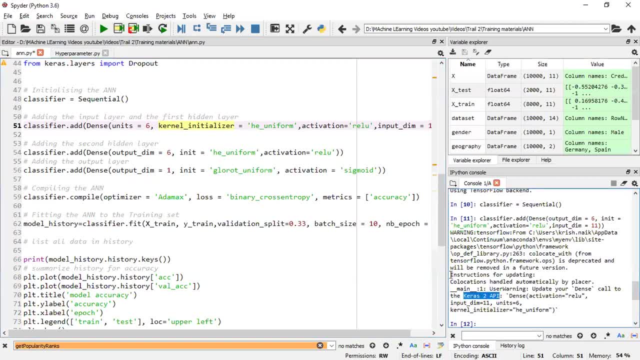 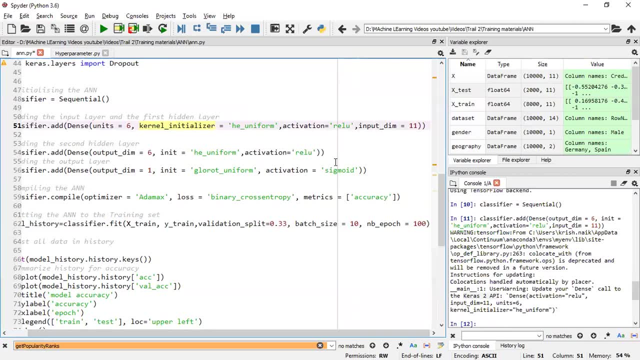 the message saying this: Keras 2.0 API. based on the Keras 2.0 API, syntax has been updated now And finally, you will be seeing that my input dimensions will be same. input dimension is almost same, only the thing that got changed is two. 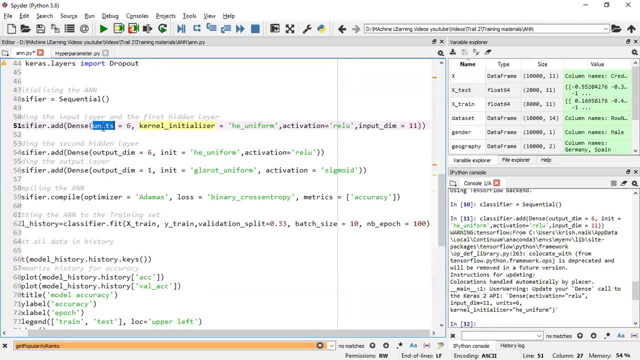 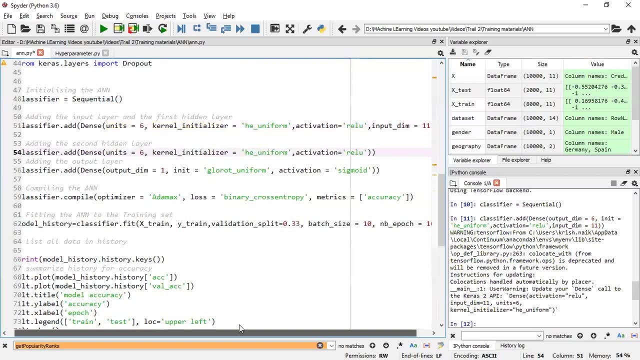 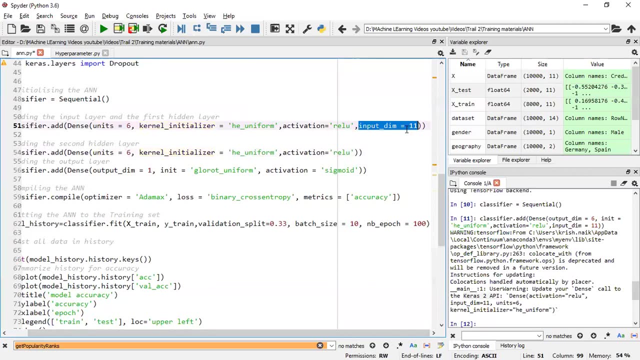 parameters, one is units and one is kernel initializer. Let me just make these changes in my other hidden layers also, And I'm currently using heUniform for ReLU because that works well. And remember guys why I've given input dimensions as level. This basically indicates that how many input 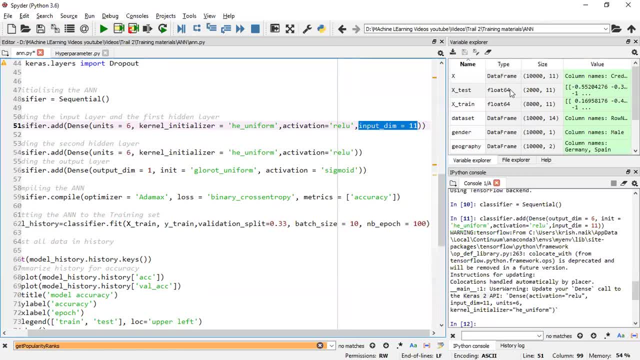 features are connected to this hidden layer. So, based on my, if I see my x train, I can see that total number of columns are 11.. So because of that, I've given my input dimension as 11.. So, in short, this creates a neural network wherein. 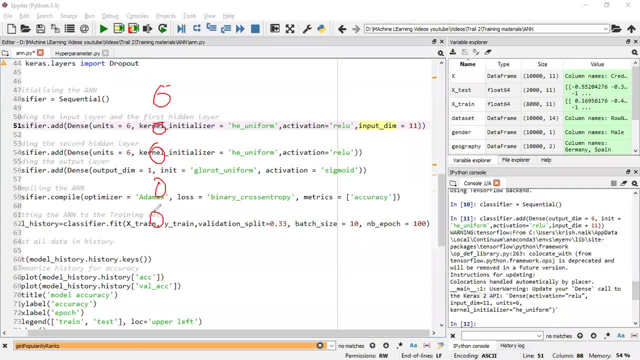 your first layer is basically having 11 input neurons. right like this. Your second layer is basically having six hidden neurons. OK, So it is seven. So, OK, It is six. Sorry, So this three and this three. Similarly, I'll add again six hidden neurons in my 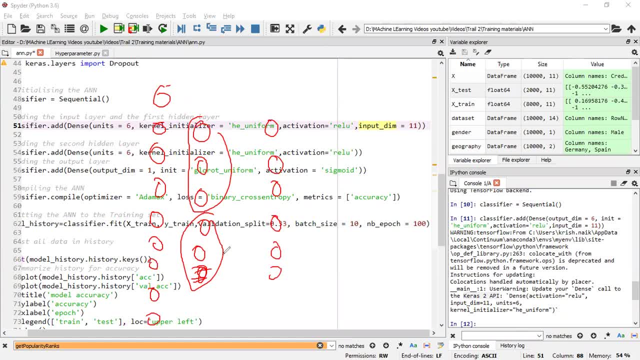 next layer, Why I'm doing this, how I'm coming to know that I have to add six. I've just put up six right now. Later, by using hyper optimization technique, I'll show you how we can come to exact solution. that how many hidden neurons I have to use. 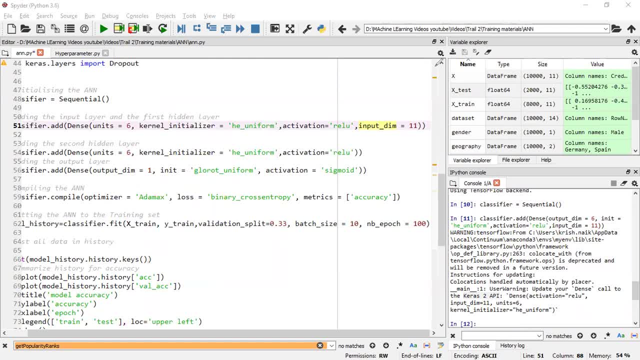 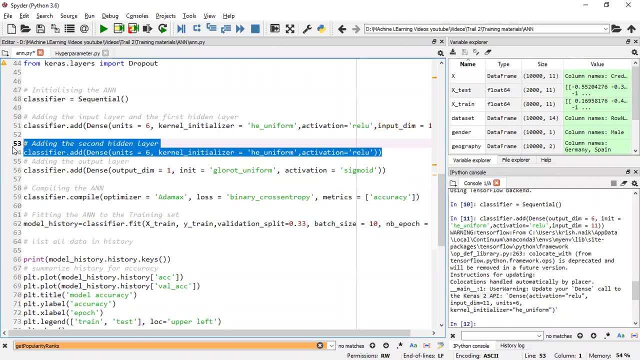 How many hidden layers I have to use. So that is what I've done in this particular first step. In the second step, I'm again adding a hidden layer with six hidden neurons. OK, So I'll just execute it. First of all, let me just execute it from scratch. 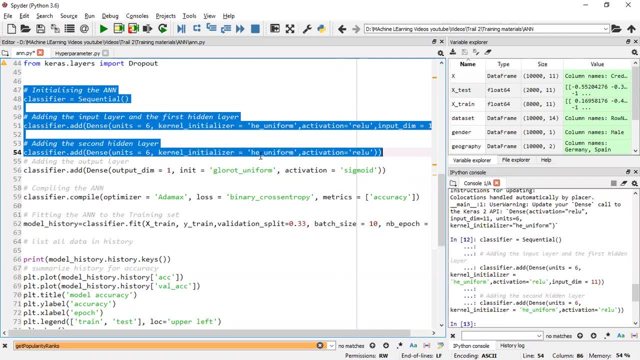 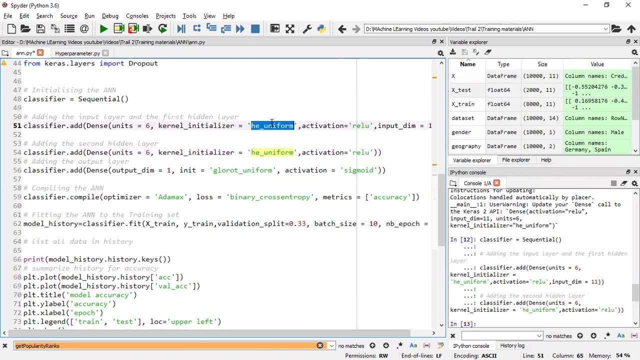 starting OK. So here again, I've used my kernel initializer as he uniform and my activation function is ReLU. If you don't know about this weight initialization parameter, please look to my videos of weight initialization in deep learning playlist. I've already explained about it. 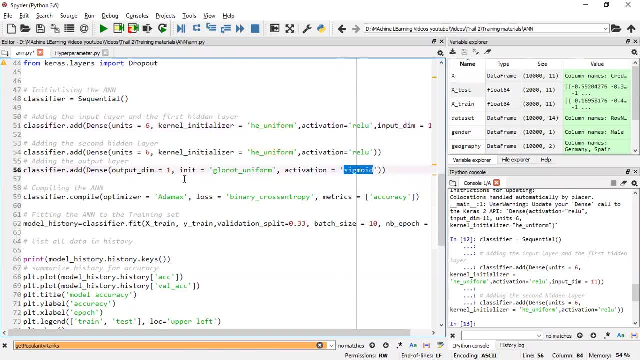 And finally, we have also discussed about sigmoid activation function. Right, And my last layer will be a one dimension. So basically, I'm happy. I I need only one hidden neuron, because this is a binary classification And based on that I will be able to predict whether, if it. 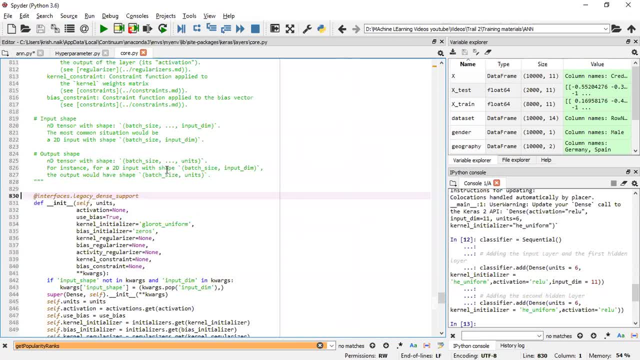 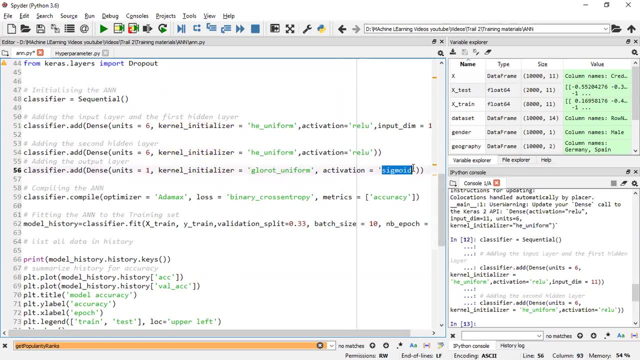 is greater than point five, I'll say that the answer will be one: OK. This answer will basically be one OK. So for that only I'm using sigmoid activation function. always remember, guys, all your hidden layer should be having ReLU or leaky ReLU, because those are the most. 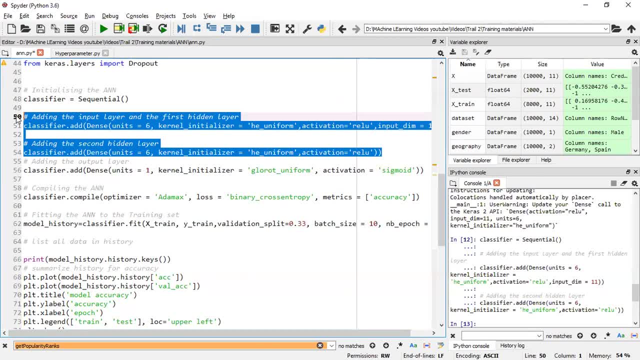 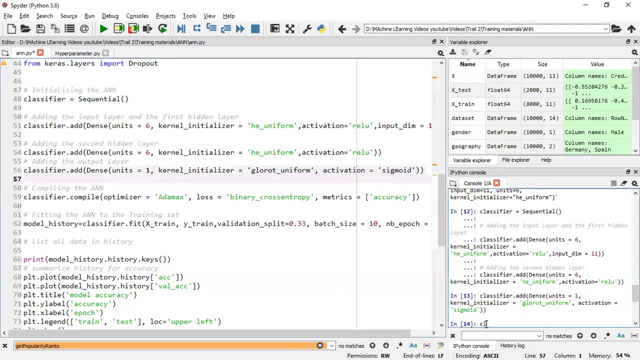 famous activation function. and ReLU prevents, you know, vanishing gradient problem issues as compared to the sigmoid. So finally, I'm going to add one neuron. So here I'll execute it. Now, if I go and see my classifier, Or summary, I see this: 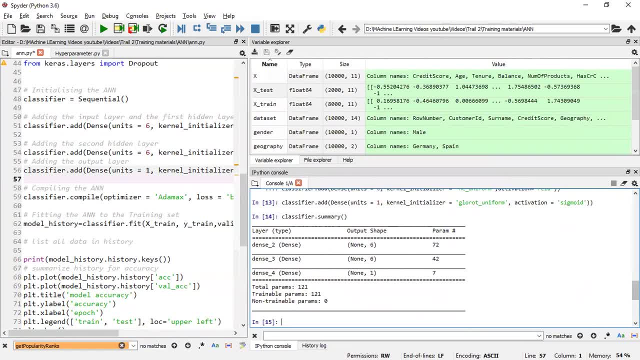 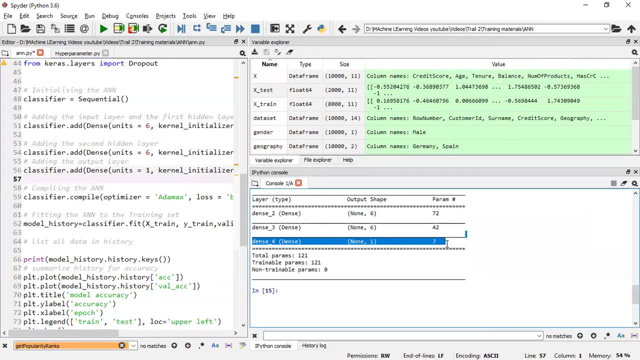 And see that it will show me the complete, Complete: How many layers I basically have, How many number of output neurons I basically have. Everything it will show and total number of patterns basically indicate that how many weights and bias parameter are there. You can also calculate it by seeing that: how many neurons. 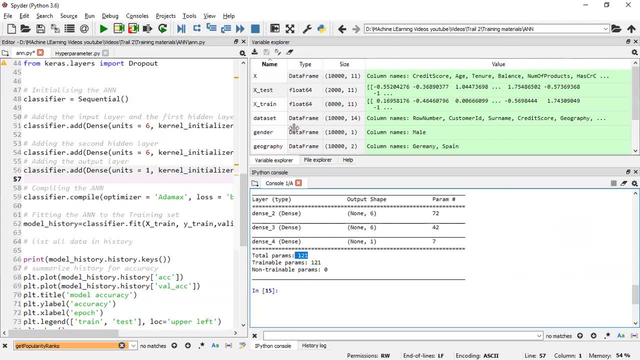 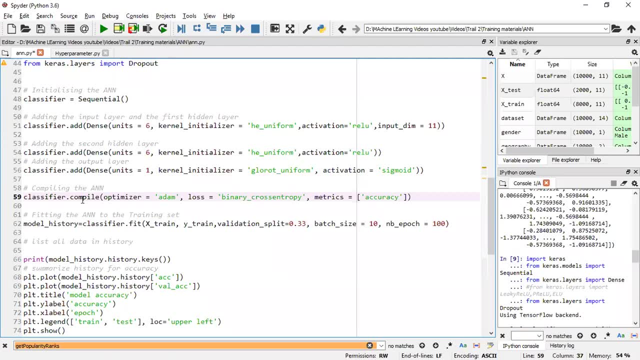 are basically there and how many number of weights that will get created. You can calculate it manually. After this, We will be compiling and I'll be providing my what kind of optimizer I'm going to use, what kind of loss function I'm going to use and what is the metrics. 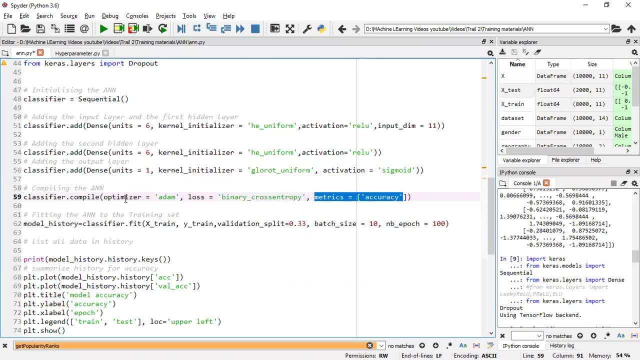 that I'm looking for Now. always remember, guys, in the first epoch, right, You know that the weights and the inputs gets multiplied, and similarly it happens in each and every layer after the activation function is applied. OK, Now final output. when you get it, then you derive your loss. 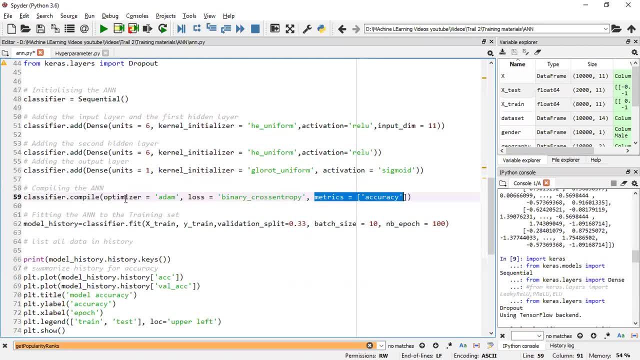 function and you create an optimizer which will reduce your loss function. right Now here I have discussed about different types of optimizers. like we discussed about stochastic gradient descent, we discussed about at a delta, we discussed about at a grad, You know, we discussed about RMS prop. 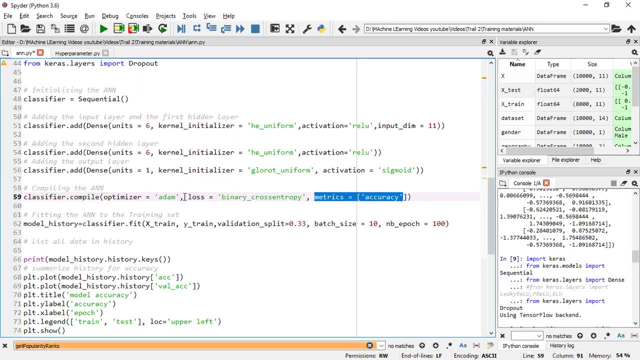 We discussed about either. currently, Adam is the best and the most popular one, So what you can do is that you can write: optimizer is equal to Adam loss. We will basically be using binary underscore cross entropy. Now, always remember, guys, whenever your output is either 0. 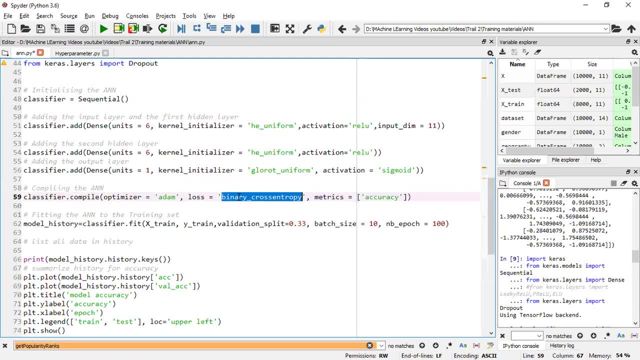 or 1, you should prefer using binary underscore cross entropy. If your output has multiple categories, then you should basically use category of cross entropy, and this information is basically given in the Keras documentation and the metrics that I'm going to use is accuracy, So let me just compile this. 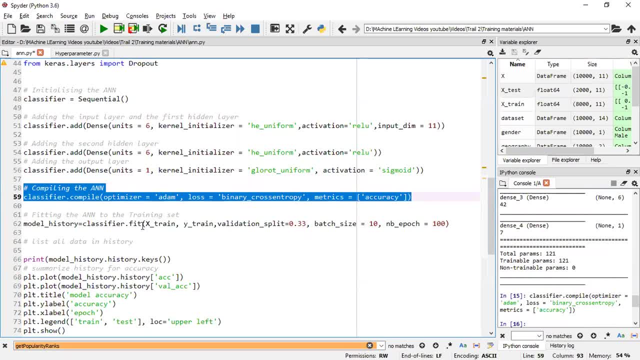 Basically I'm setting up my optimizer and finally I'll do the fit where I'll say that take my extreme white train validation split. I'm also going to take validation split so that I can test my data set separately, but test this model separately for the 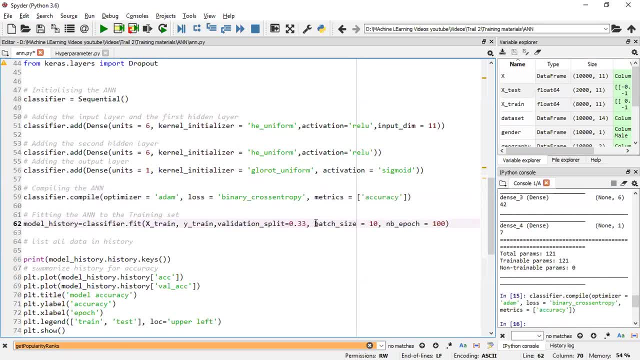 you know for for the test data set and then I will set my bath size to 10.. I hope everybody knows why we use bath size. bath size is specifically used so that the computation power becomes less. More amount of records You don't have to load at just one time. 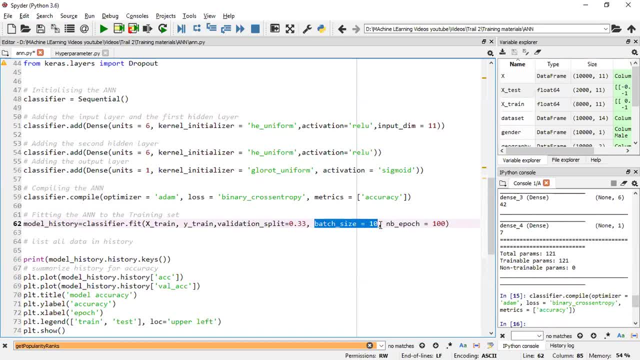 Your RAM will be pretty much free and you'll be able to run this program in your laptop. And then this is basically your number of epochs. Now let me just execute this. Let me just execute this Now. after you've seen this, you'll be seeing that your 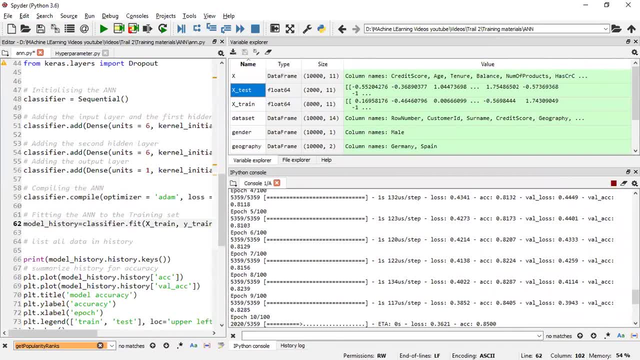 epoch will be starting and total number of epochs that I'm going to run is 100.. You can see over here the accuracy is increasing. It has come to 86. But using the right kind of Internal initializer, which is your weight initialize and other. 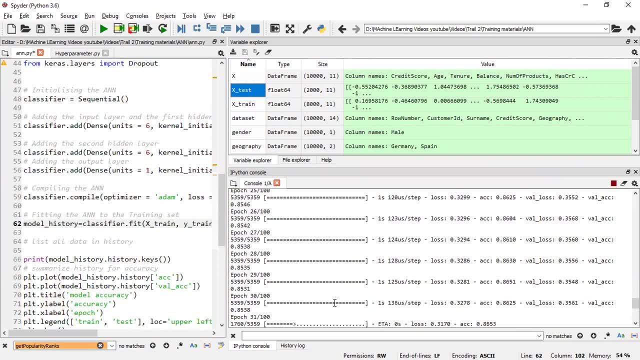 parameters. it is going to take some time, approximately five minutes or three to four minutes, And then I'm just going to pause this video. I'm just going to fast forward it. till then I'll just pause it and I'll continue once the training has got over. 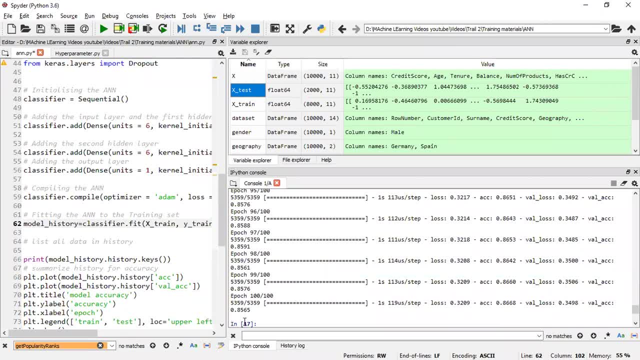 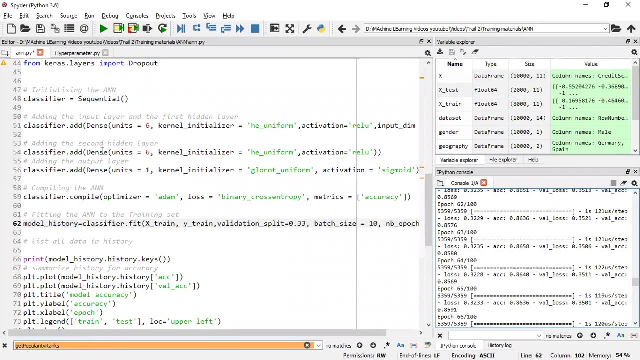 So 98 epochs has got completed and this is my 100 epoch. Now, after 100 epoch, you can see that your accuracy, training accuracy, is 86 percent. Your validation accuracy is also somewhere around 85 percent, guys. So remember, by just selecting the right kind of initializer and by 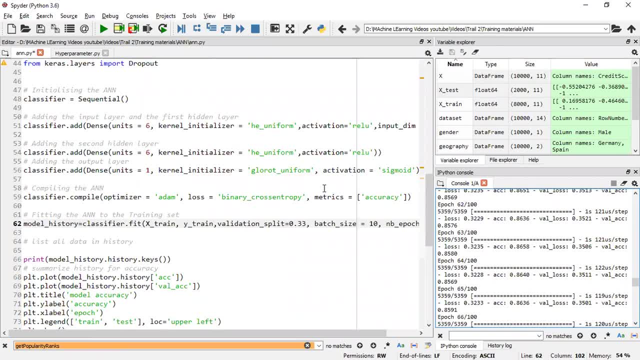 just using a simple neural network you are able to get 86 percent. But just imagine if you don't select this parameters perfectly, which I have already tried. you just try to select some other parameters for kernel initializer right Suppose kernel initializer, you can also consider uniform. 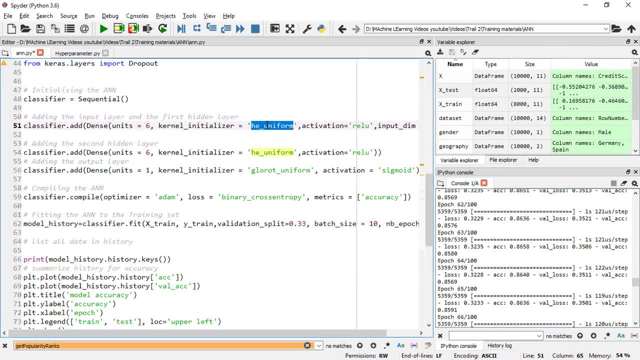 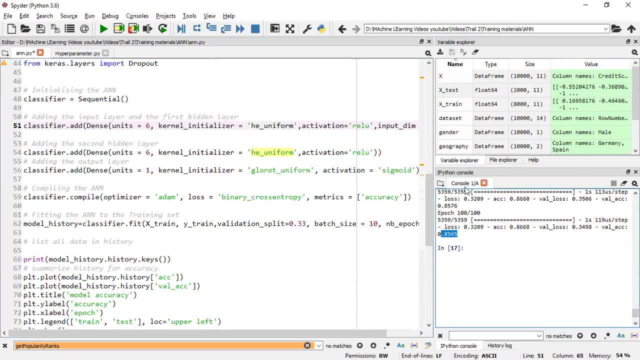 OK, At that time I saw that the accuracy had decreased to 82 percent. Right, So this after training, you can see that I have better, got an accuracy of somewhere around 86 percent. Now what I'll do is that I'll try to test it for my training. 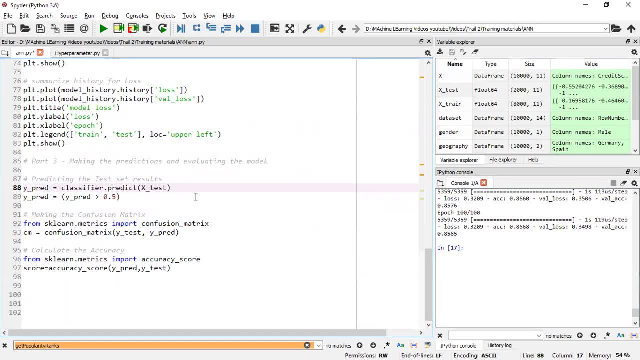 data, sorry, test data. Now what I'll do? I'll just say classified or predict on X test and finally I'll say: whichever is greater than point five, consider it as true or false. And then I'll be using my confusion matrix, Confusion matrix. for this I'll be importing from the confusion. 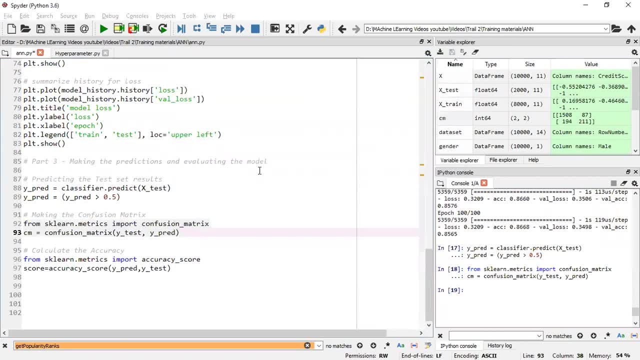 matrix library. This is how my confusion matrix looks like. If I go and see my accuracy score for the test data. and this is my score, Let me see. Let me see my score over here. So it is somewhere around 85 percent guys. 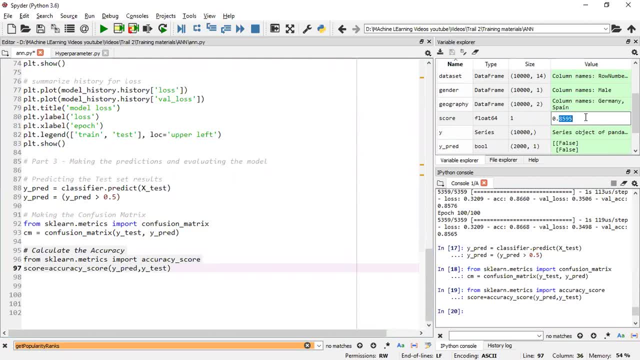 The training accuracy is almost same, The validation accuracy is almost same and your final accuracy of your test data is almost, also almost. This is a perfect way of doing it, And what I will do is that I will try to increase the number of units. 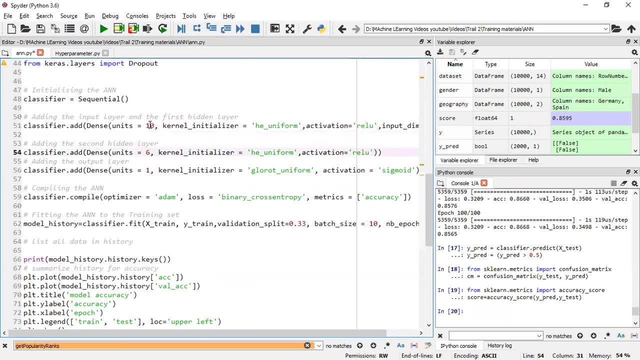 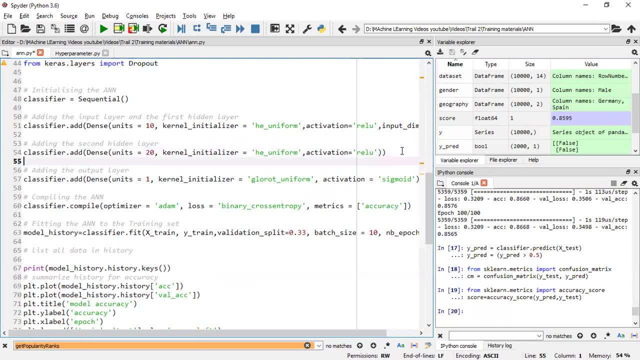 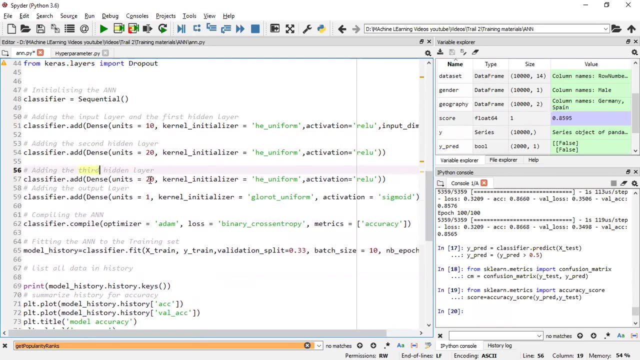 Let's see if I try to increase the number of units, that is, my number of hidden neurons, to try to increase one more layer, Let's, let's, let's just increase one more. Let's say that, adding the third hidden layer. OK, And here? 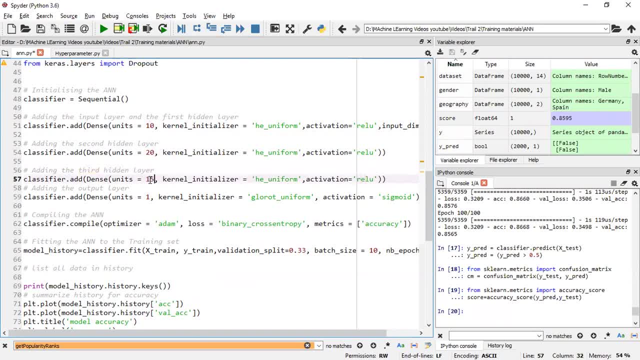 OK, let me just take it as 15 hidden neurons. OK, So here also I'm going to use activation function. Instead of he uniform, I'll use he normal. This is also another way to initialize that works well with ReLU, Looks well with ReLU. 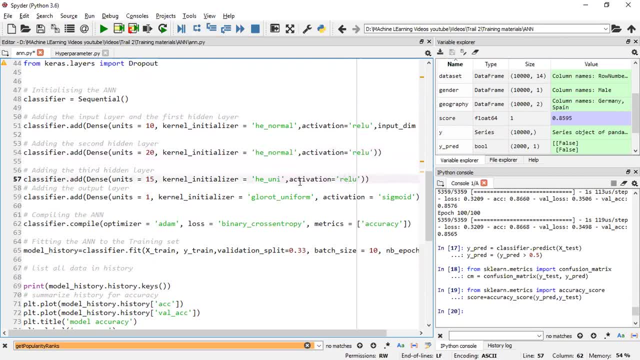 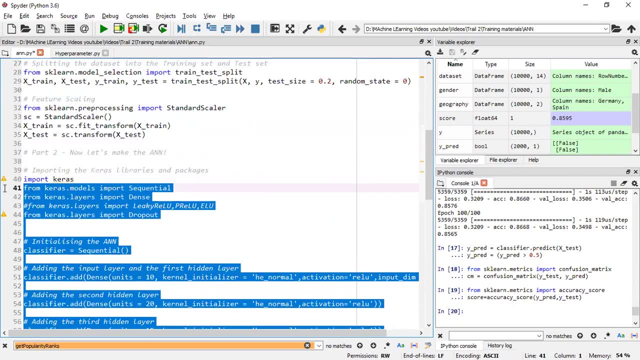 From where I'm getting this information that I already showed you, from the garage documentation. You can basically try different, different things. I will execute everything till here, from here, So from here, I'm going to execute it again. Again, it will take some time for execution. 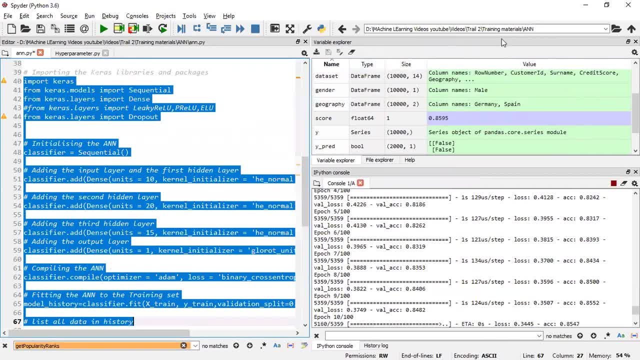 I'll just pause the video and I'll just come back when the epoch is somewhere around the 90th epoch. So 80 epoch has been completed. Another 16 more epochs. See how quickly the things are happening and you can observe something: that accuracy is also increasing, right. 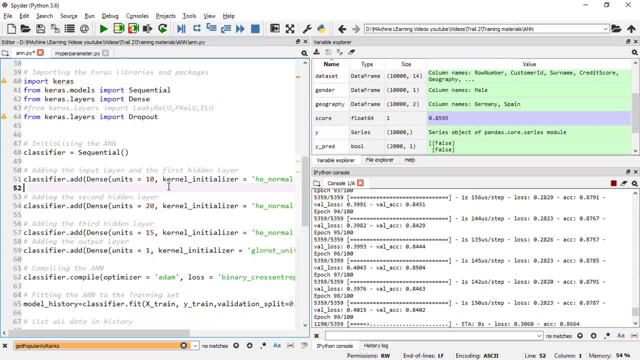 When I use the previous combination- and again this is from research guys- they have told that use this particular mechanism wherein, if you are using ReLU, use this kind of initializer. it will work well. So I've also done a lot of permutation and combination, But what I observed- the validation increases decreased. 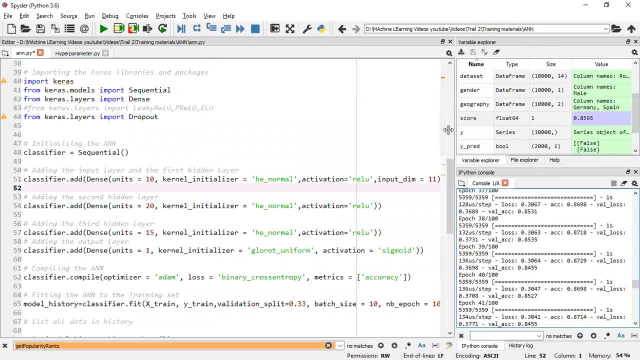 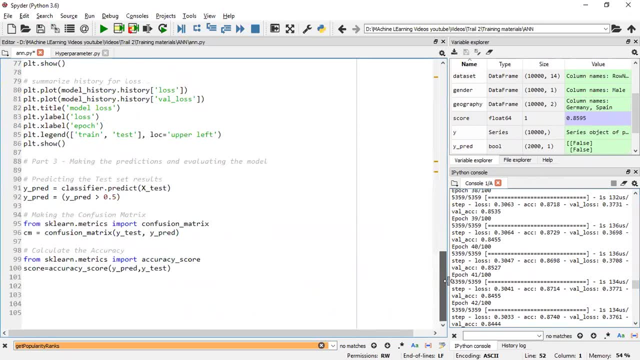 from the previous time, But let us see for the test data what accuracy it brings. So currently, my previous model score was 85, somewhere around this can be considered 86 percent. Now what I'll do? I will just execute this, all things Now. 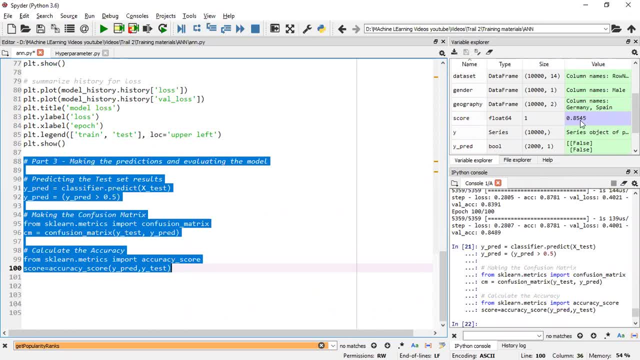 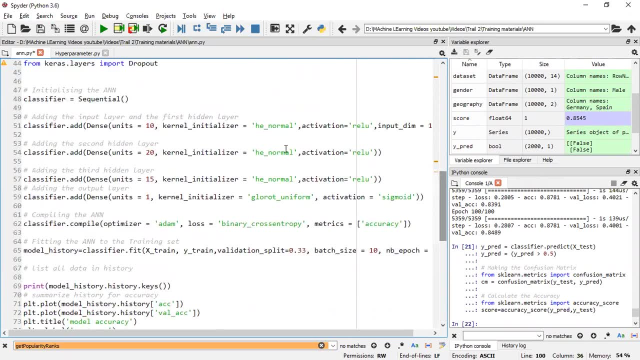 Yes, It is almost similar. It is basically having 85 percent. Now, if you want to still more increase accuracy, guys, I'm telling you, don't do it as an overfitting, don't create more multiple layers. Let us just try to add dropout. 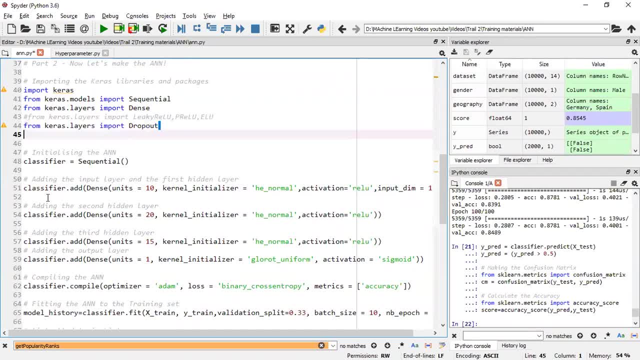 Now, if I create a deep neural network, what I can do is that I can basically create a dropout layer. So let me just write it out: If a classifier dot add- and I hope everybody knows what is dropout, If you have a deep neural network you can basically apply. 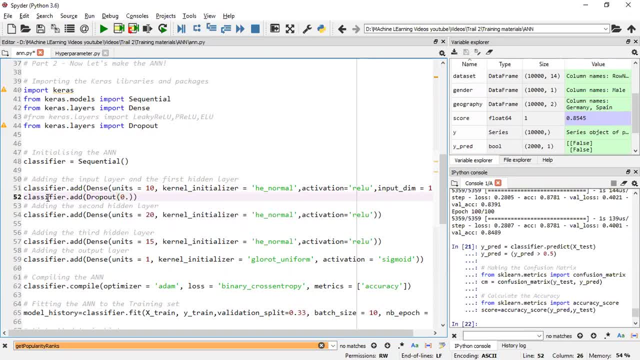 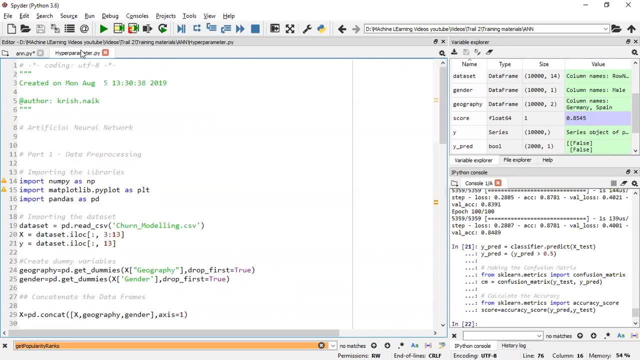 dropout, with some dropout ratio like 0.3.. I've just taken randomly, But later on I'll try to find out all these values by using hyperparameter optimization. See, your code is also ready. I'm just working on it and I'll show it to you how to do it. 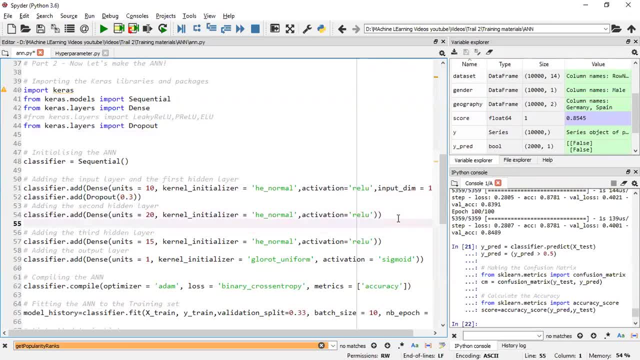 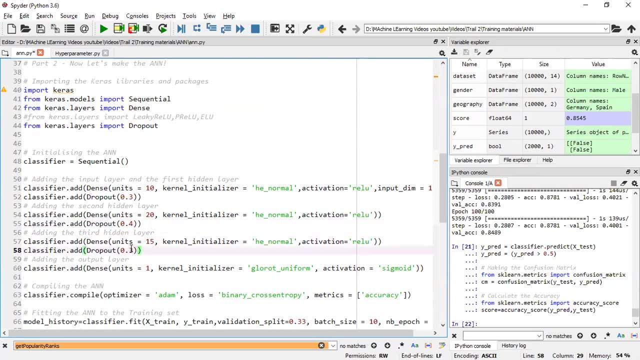 OK, So, but just understand over here, right now I'll just apply dropout every way. So suppose I'll apply 0.4 here and the number of neurons are a little bit less. I'll just apply point after applying dropout. let's see whether. 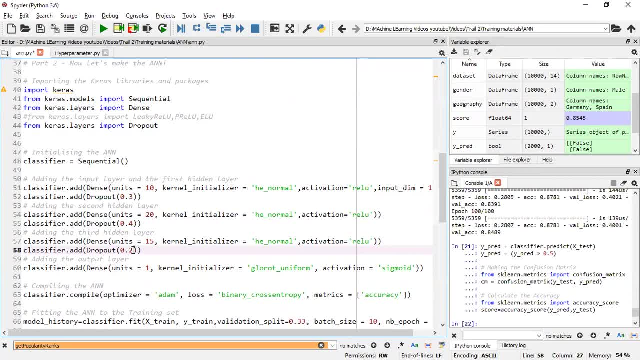 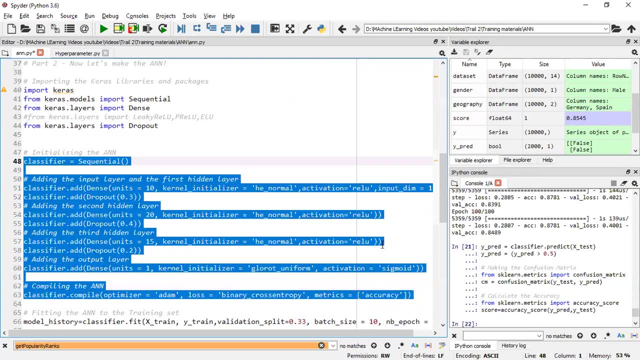 this will increase because I just have 10,000 records, guys, but in most of the scenario you'll be getting a million of records to work with. Let's again compile from the starting and do the fit again. What I'm going to do is that I'm going to execute from here. 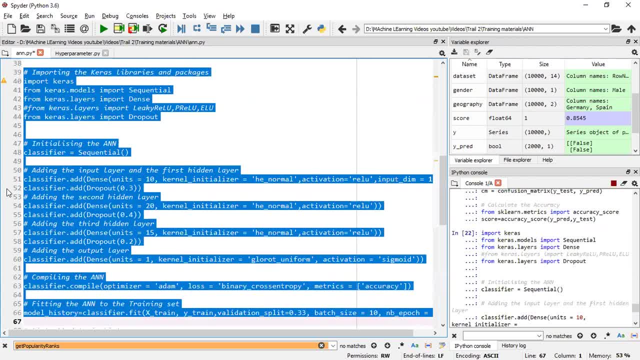 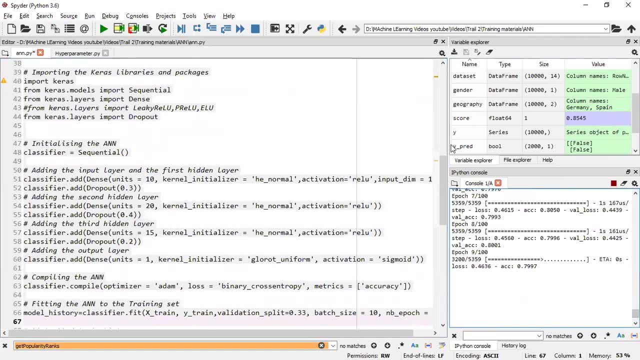 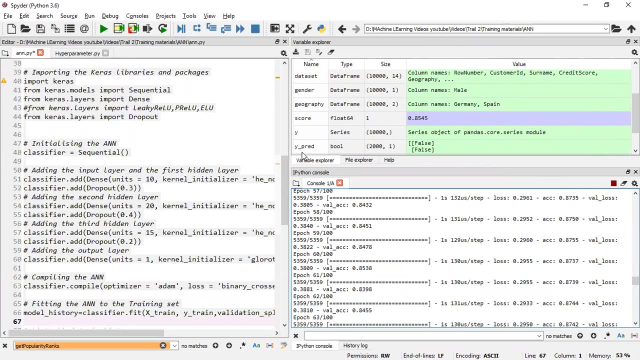 And I'll execute till here All the combinations you should basically try and should try to see whether they are improving things or not. Oh, has it started? Yes, it has started again. It will take another three minutes, so I'm just going to pause the video and come back in the 90th iteration. 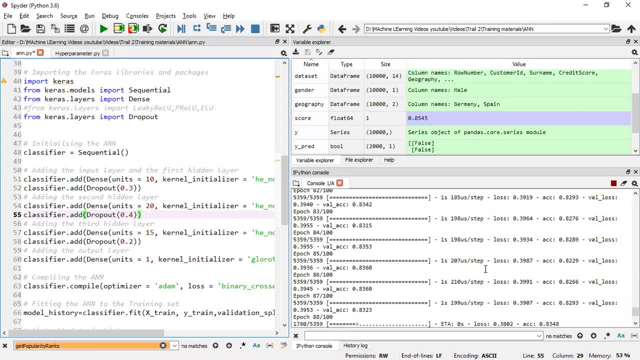 So 85 epoch is about to complete. yes, 86. now 10 more epochs. But what we observe here, the accuracy has been still in 82 percent. by using the previous techniques, by using without dropout, At that time we were able to get 86 percent. but don't just. 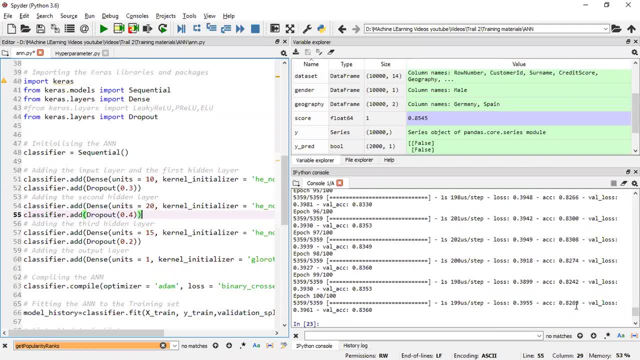 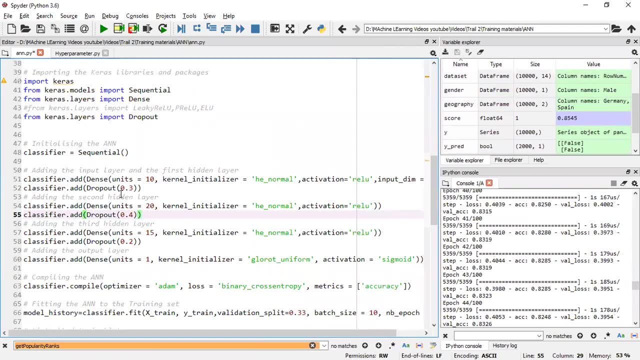 consider the guys whether this accuracy, if it is coming down, that does not mean that it is having a bad accuracy. See, Oh Scenario may be leading to overfitting and underfitting. dropout also plays a very good role. If you, if you, if you don't know about dropout, I've already 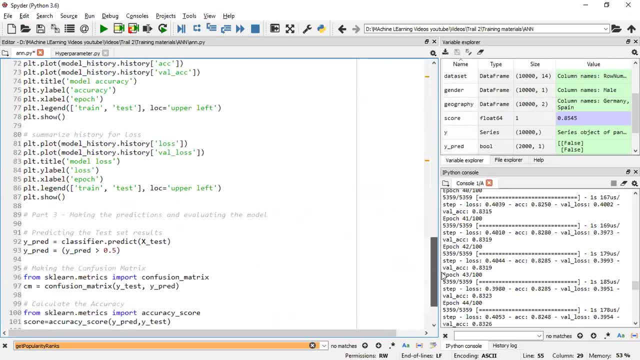 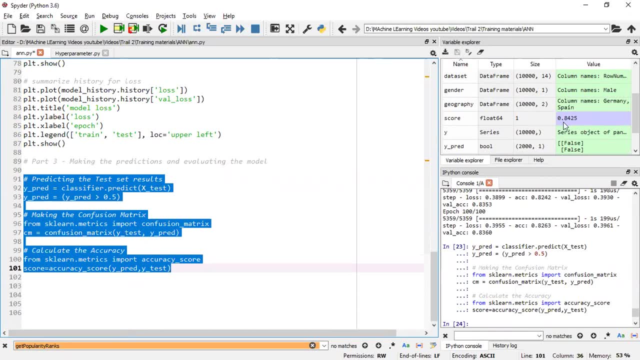 created a video in my deep learning playlist and you'll understand the importance of dropout by by seeing that video. Let me just go and predict it for a test data again Now you can see my test score has just come down by one percent that I think you should try to apply dropout for very. 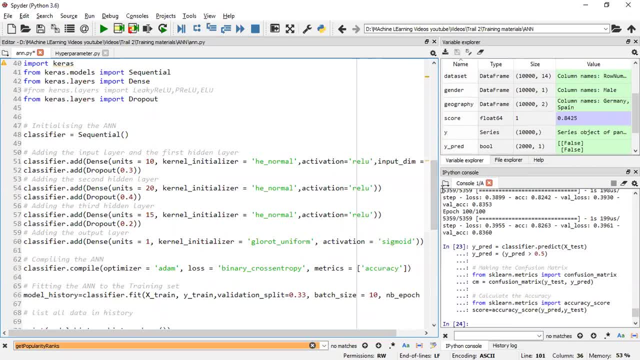 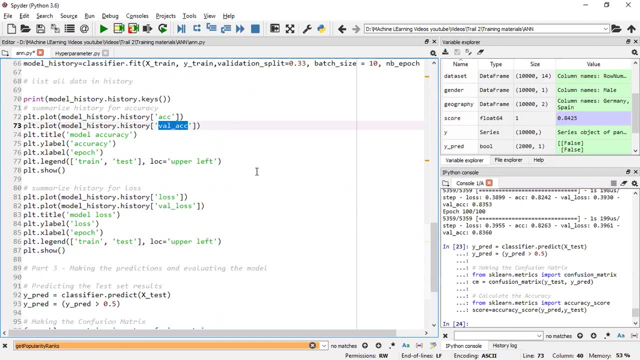 very deep neural network, because that will give you the right type of combination for testing the data. So this was all about the artificial neural network creating from scratch. This, to quote, basically helps you to see how your validation accuracy was going down, coming up in the graph wise. 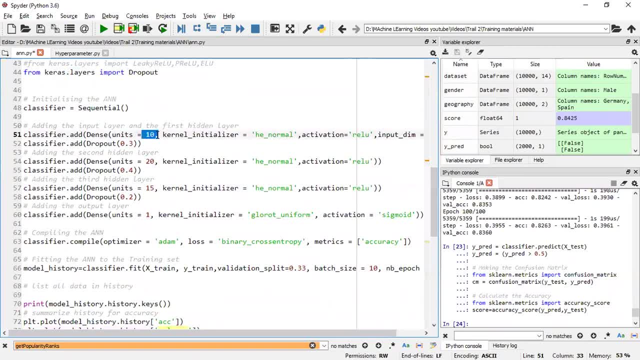 The main thing is, guys, that we need to know how to initialize this. how many number of layers is suitable for my neural network? How many number of hidden neurons? or should I take which activation function is good, Right? So we should try to do this combination by using a hyper.